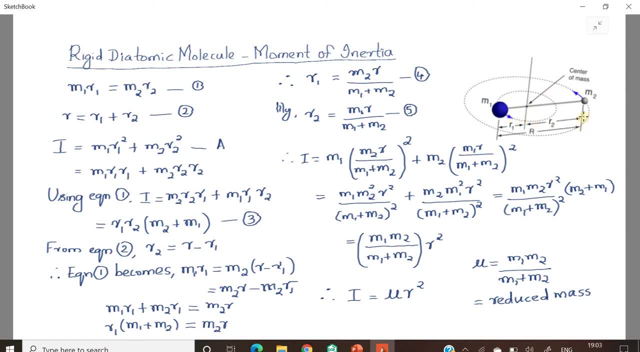 Let distance be d2.. Let distance be d1.. Let distance be d2.. r1 and r2 from the center of mass. So the center of gravity is defined by m1. r1 equals m2, r2.. If r is the equilibrium bond length, then r equals r1 plus r2.. Now we are considering the molecule. 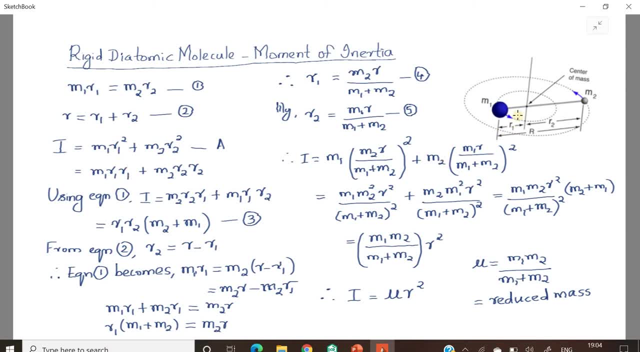 as one in which the two masses are joined by a rigid bar of length r, so that the molecule becomes a rigid rotator or a rigid rotor. So the moment of inertia for such a rigid molecule is given by: i equals m1 r1 square plus m2 r2 square, which can also be written as m1 r1- r1 plus m2 r2 r2.. 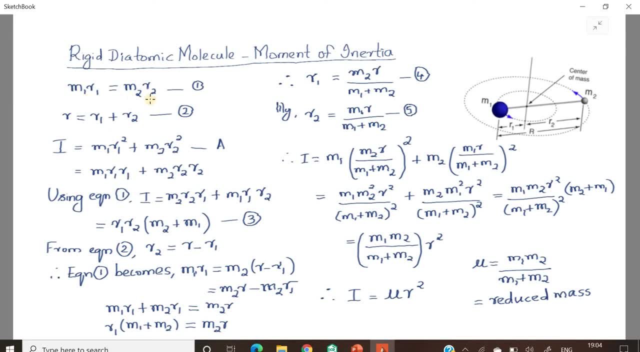 Now, according to equation 1, m1 r1 equals m2 r2.. So in equation a we write m2 r2 instead of m1 r1 and m1 r1 instead of m2 r2.. Therefore i equals m2 r2- r1 plus m1 r1- r2.. Here r1 and r2. 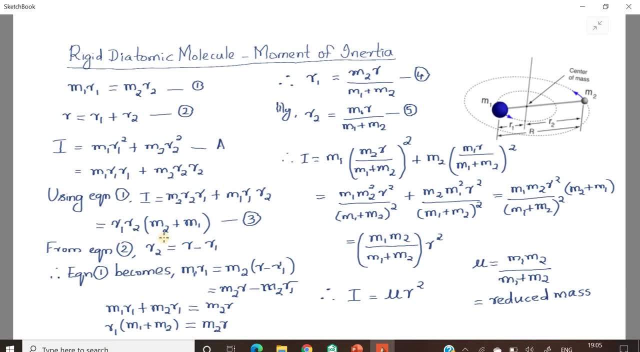 is common. so that is equal to r1, r2 into m2 plus m1.. In equation 2, r equals r1, r2 plus m2, r1. plus R2. or we can write: R2 equals R minus R1.. Substituting the value of R2 in equation 1, we: 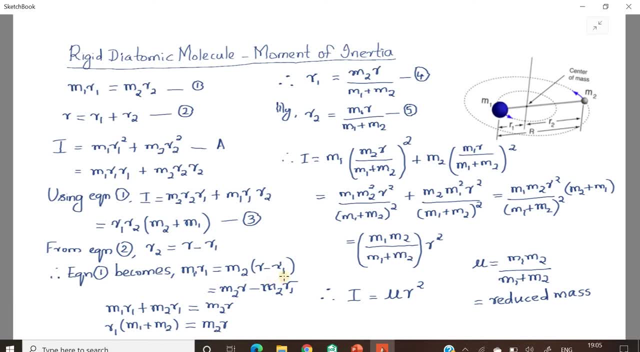 can write M1 R1 equals M2 into R minus R1, which is equal to M2 R minus M2 R1.. On rearranging, we can write M1 R1 plus M2 R1 is equal to M2 R or R1 into M1 plus M2 equals M2 R. 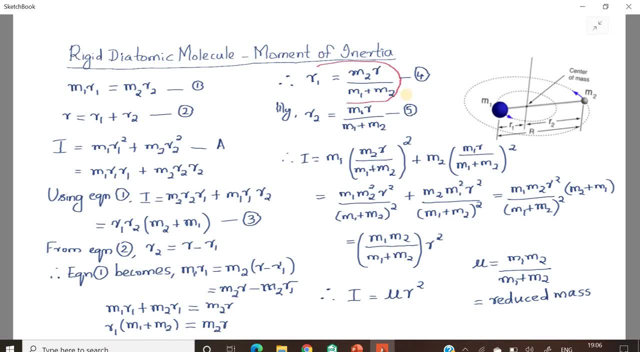 Therefore, R1 is equal to M2 R by M1 plus M2.. Similarly, using this equation R equals R1 plus R2 or R1 equals R minus R2, we can obtain the value for R2, that is, R2 equals M1 R by 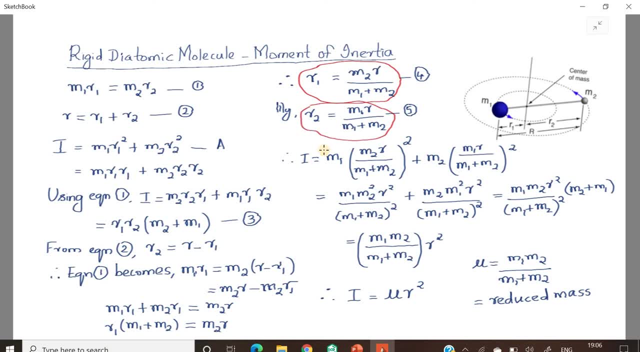 M2, R1.. M1 plus M2.. Now in equation A we substitute the values of R1 and R2, that is, I equals M1 into instead of R1 square. write M2- R by M1 plus M2, the whole square plus M2 into instead. 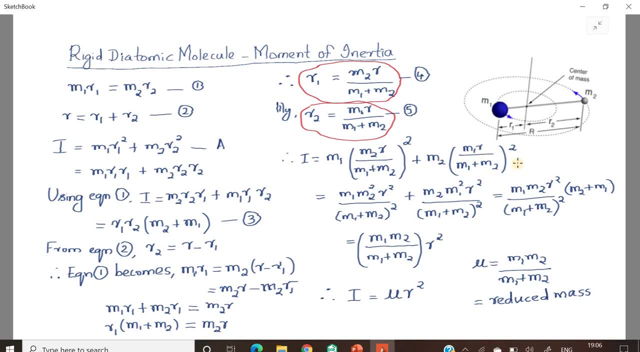 of R2 square. write M1- R by M1 plus M2, the whole square, which is equal to M1 M2 square. R square by M1 plus M2, the whole square. So here in both terms M2, M1 and R square is common, So that is equal to M1 M2- R square. 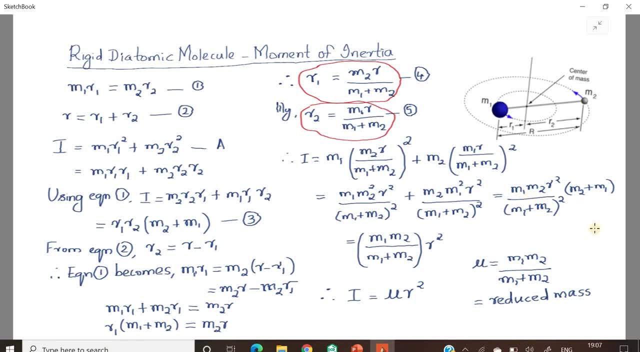 by M1 plus M2 the whole square into M1 plus M2.. So if we cancel off 1 M1 plus M2, we have the moment of inertia. I equals M1 M2 by M1 plus M2 into R square, which can be simplified as I equals mu R square, where mu equals M1 M2. 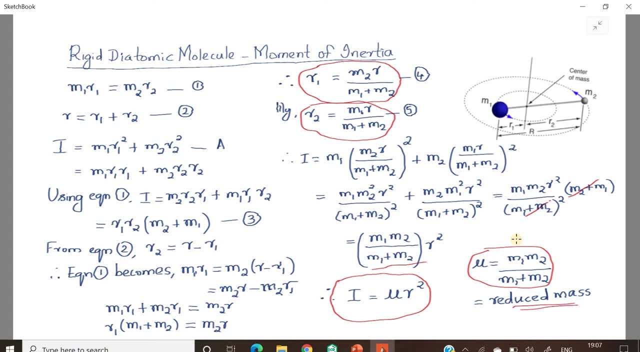 by M1 plus M2, which is called the reduced mass of the molecule. So we have obtained the equation for moment of inertia of a rigid diatomic molecule which is: I equals mu- R square, Where mu equals M1, M2 by M1 plus M2 and is known as the reduced mass of the molecule. 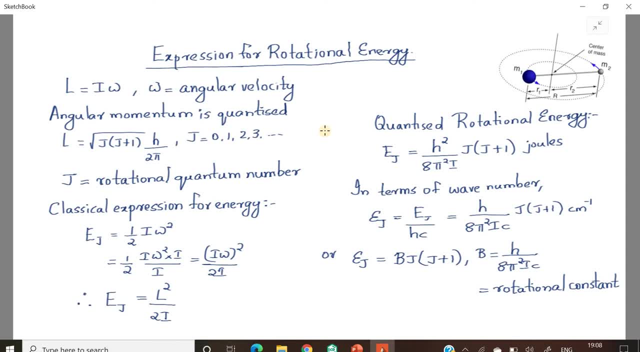 Next step is to derive the expression for rotational energy of the diatomic molecule. So we have considered the rotation of a diatomic molecule. The angular momentum is given by L equals I, omega, where I is the moment of inertia and omega is the angular momentum. 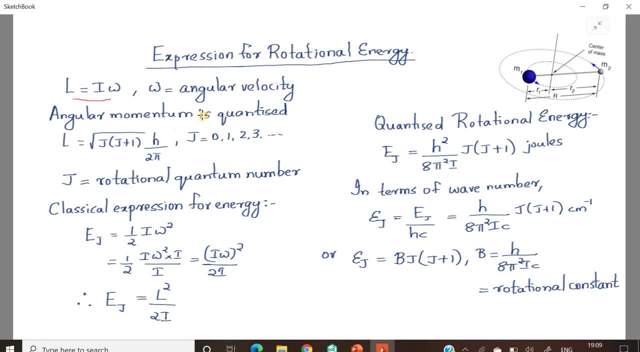 The angular momentum is quantized and its values is given by: L equals root of J into J plus 1 into H, by 2 pi, where J equals 0,, 1,, 2, 3, etc. and is known as the rotational quantum number. 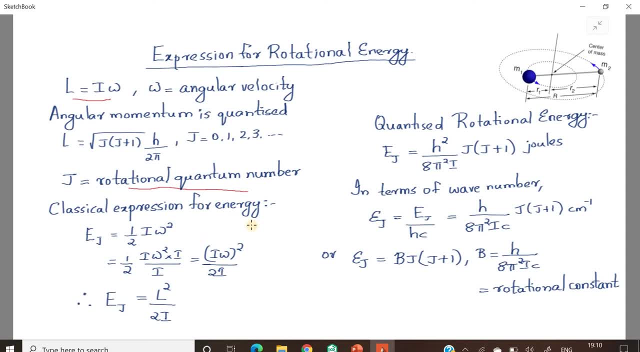 The classical expression for energy is given by rotational energy is given by: EJ equals half I omega square, which can also be written as half I omega square into I by I, which is equal to I omega, the whole square by 2I. I omega is L, the angular momentum. 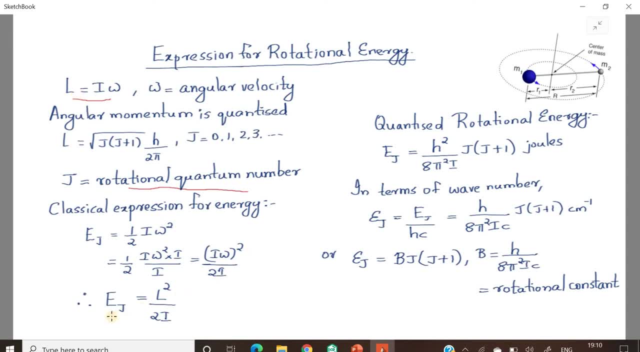 So instead of I, omega, the whole square, we can write L square. So E equals L square by 2I. Now if we substitute the value of L in this equation, which is L is equal to root of J, into J, plus 1 into H, by 2 pi. 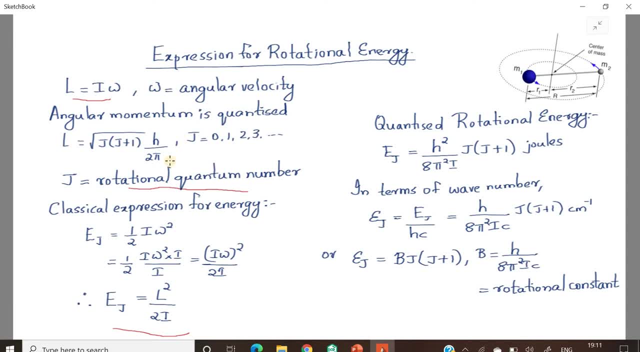 Therefore, L square becomes H square by 4 pi square into J, into J plus 1.. If we substitute that we will have the quantized rotational energy of a diatomic molecule, that is EJ, equals H square by 8 pi square, I J into J plus 1 joules. 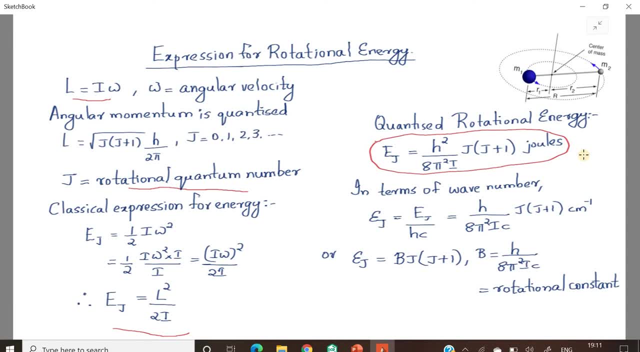 The energy is in joules. E equals H square by 8, pi square I J into J plus 1.. Where H is the Planck's constant, I is the moment of inertia and J is the rotational quantum number. Usually we express the energy in terms of wave number. nu bar. 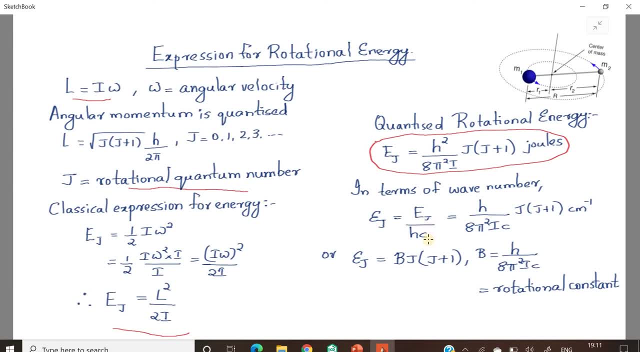 So epsilon J equals EJ by H into C. H is the Planck's constant, C is the velocity of light. So in terms of wave number we can express the rotational energy as epsilon J equals H by 8 pi, square I, C, J into J plus 1.. 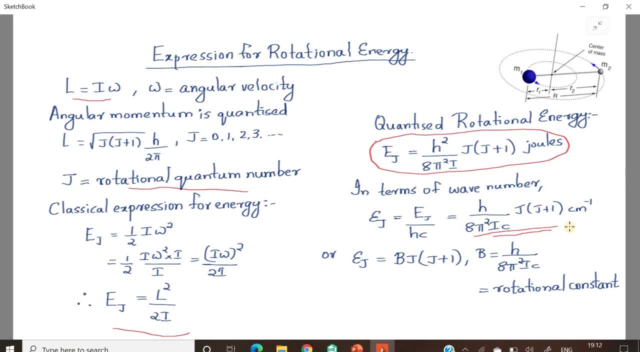 This can be simplified as epsilon J equals BJ into J plus 1, where B equals H by 8 pi square I C, and that is known as the rotational constant. So we have defined a new term, B, which is called the rotational constant, whose value is given by: B equals H by 8 pi square I C. 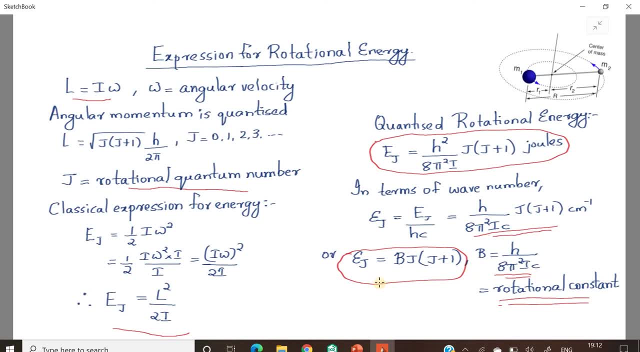 So these two equations are important. One is the equation for rotational energy. In terms of joules, it is: E equals H, square by 8 pi, square I J into J plus 1.. In terms of wave number, we have epsilon: J equals BJ into J plus 1, where B is the rotational constant and its value is given by H by 8 pi square I C. 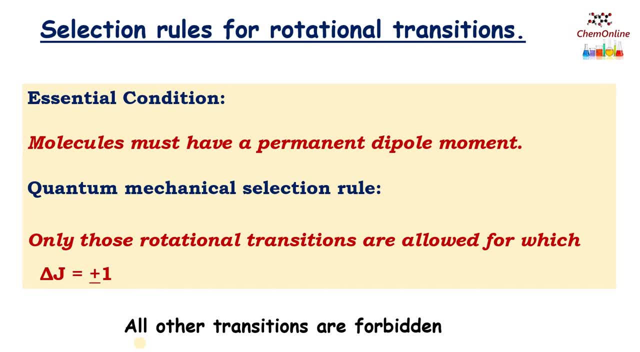 We have seen the moment of inertia and rotational energy of a diatomic molecule. Next is about the selection rules. We have already seen that only molecules with a permanent dipole moment will produce a rotational spectrum, and that is the most essential condition. By absorbing microwave radiation, the molecule will undergo transitions between the rotational energy levels. 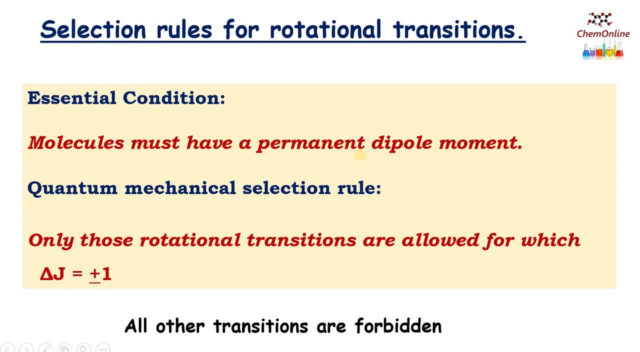 But all possible rotational transitions are not quantum mechanically allowed transitions. So there is a selection rule which determine which transitions are quantum mechanically allowed, Which can be stated as only those rotational transitions are allowed for which delta J equals plus or minus 1.. This is the quantum mechanical selection rule. 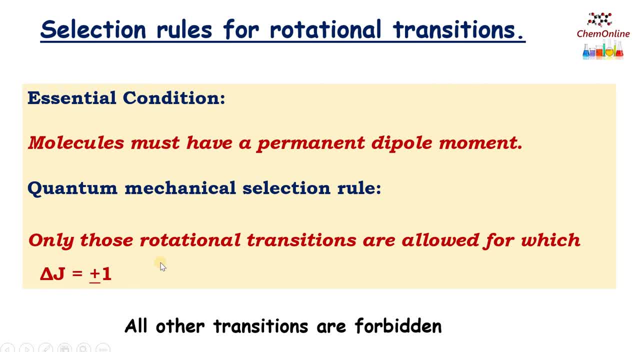 That is, only those rotational transitions in which the rotational quantum number J changes by one unit are allowed, and all other transitions are forbidden. This is a selection rule for rotational spectroscopy. So we have two conditions. The first and the foremost condition is that the molecules must have a permanent dipole moment. The second one is: 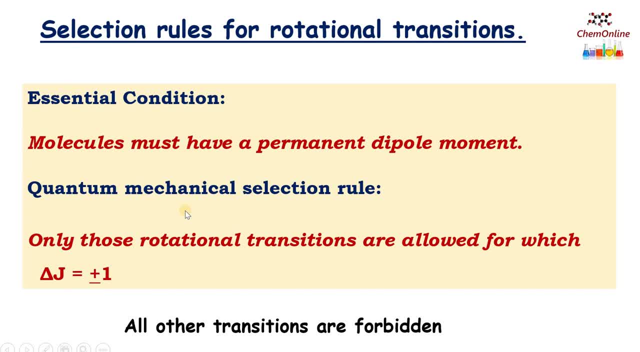 the selection rule based on quantum mechanics, which states that only those rotational transitions are quantum mechanically allowed for which delta J equals plus or minus 1. where delta J is the change in the rotational quantum number, J can change by only one unit Plus. sign denotes: 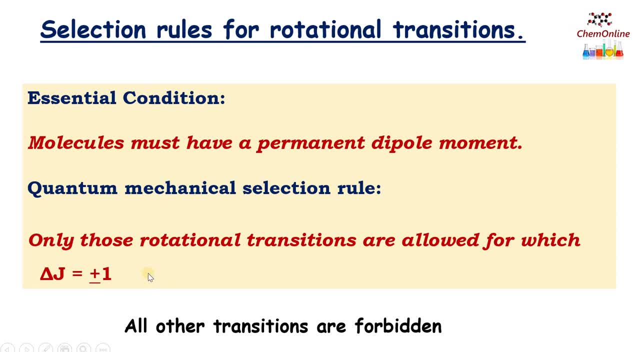 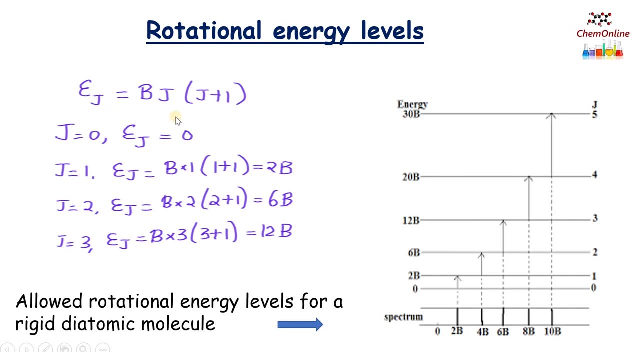 an upward transition by absorption of energy and minus sign denotes the downward transition by emission of energy. So delta J equals plus or minus 1 and all other transitions are forbidden. The rotational energy in terms of wave number is epsilon J equals b J into J plus 1.. If we put 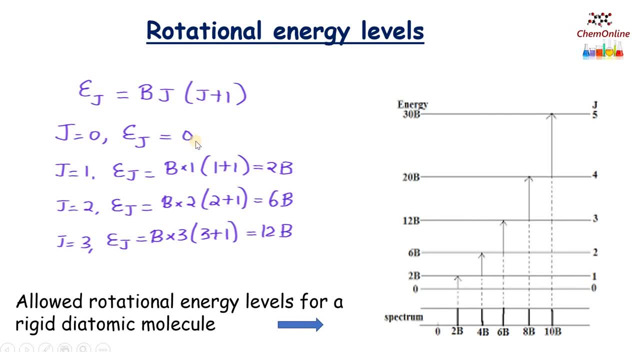 J equals 0, epsilon J equals 0.. For J equals 1, epsilon J equals 2 b, For J equals 2, epsilon J equals 6 b, and for J equals 3, epsilon J equals 2 l, b and so on. So this is represented in this. 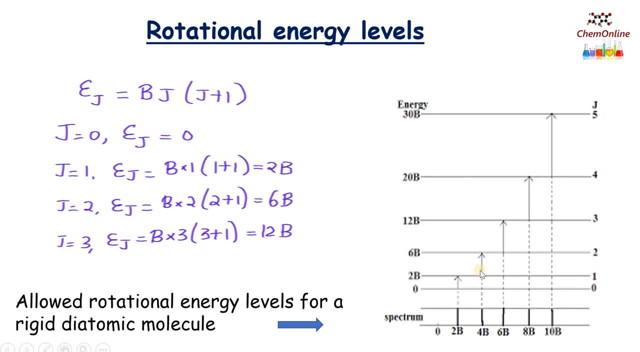 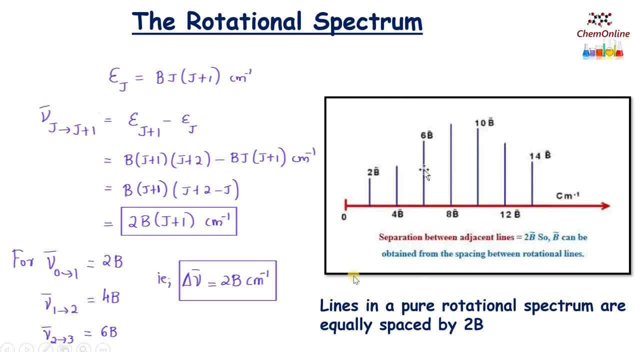 rotational energy level diagram. These are the allowed and the forbidden Rotational energy levels for a rigid diatomic molecule. Now consider a transition from the Jth level to J plus 1th level. So the energy difference between the two levels is given by epsilon J plus 1, minus epsilon J equal to b, into instead of J. 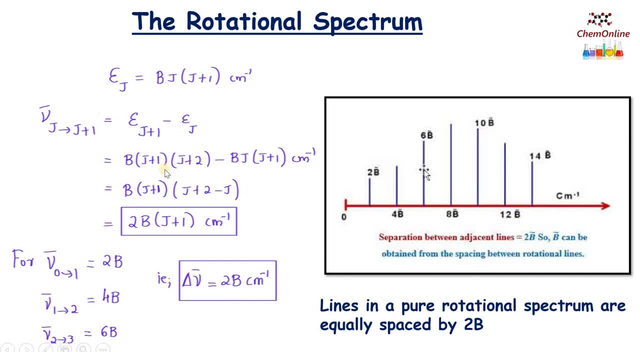 write J plus 1 because it is a J plus 1th level, So b into J plus 1 into J plus 2 minus b, J into J plus 1. The difference can be seen to be 2 b into J plus 1 centimeter inverse. 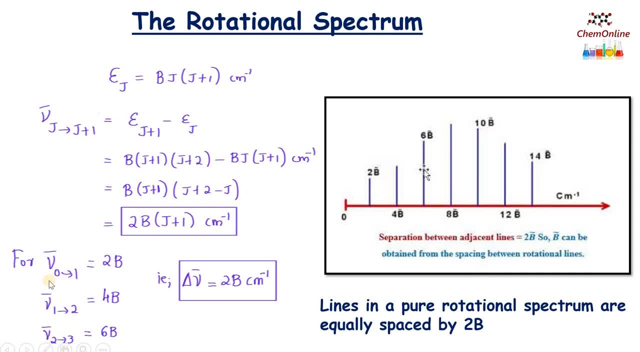 Now, if we consider the first transition, that is, from the ground state, J is equal to 0 to the first state, J equal to 1.. J equals 0. here we will get 2 b. Now the next transition will be from: 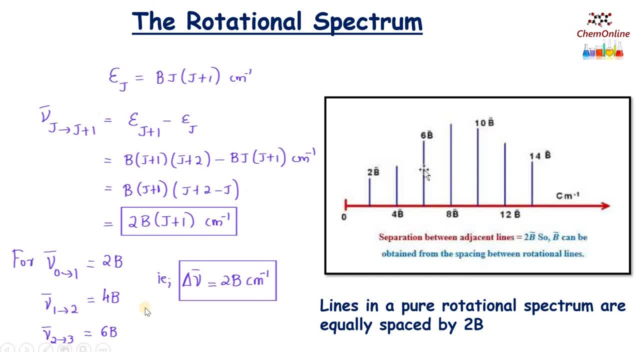 J equals J equals 1 to J equals 2, because delta J can be only plus or minus 1.. So J equals 1 to J equals 2 will have 4 b. Similarly, for J equals 2 to J equals 3, we will have 6 b. Now it goes. 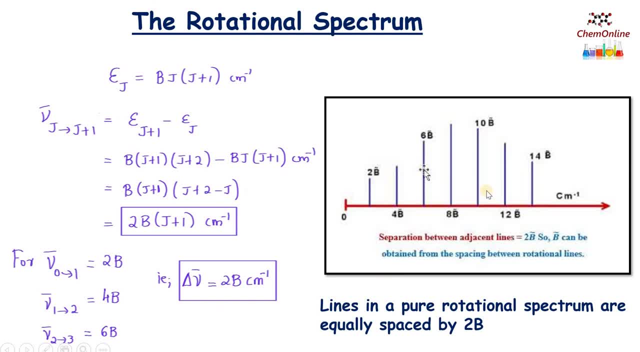 like this: That is 2 b, 4 b, 6 b, 8 b, 10 b, etc. So from this we can see that the separation between the adjacent lines is constant, which is equal to 2 b centimeter, inverse That is.